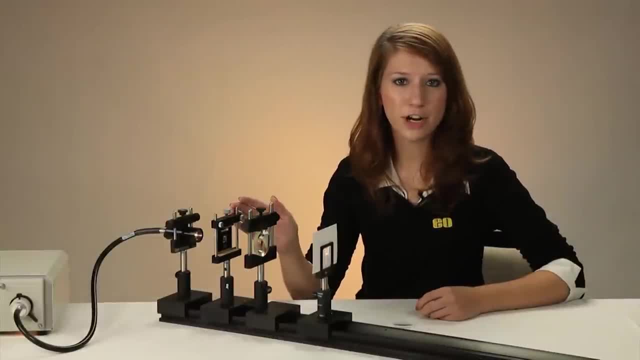 In this setup, our object is a USAF resolution target and the lens has a 50mm focal length. If we call the distance from the object to the lens z, the distance from the lens to the image plane, z- prime, and the focal length of the lens f, we can use this equation to: 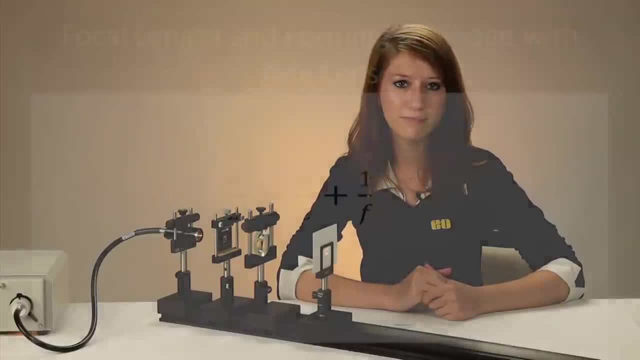 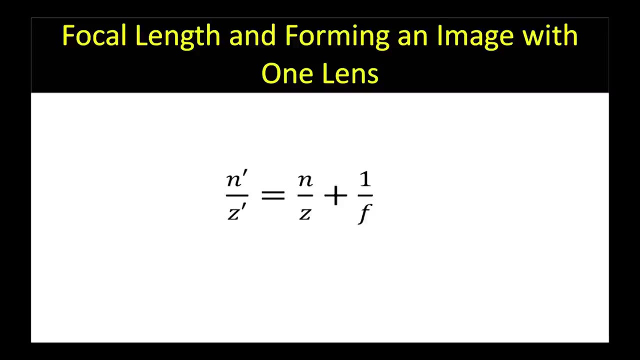 determine where the image will form or what focal length lens we need. In this equation, n prime is the refractive index of the medium between the lens and the image plane, and n is the refractive index of the medium between the object and the lens. 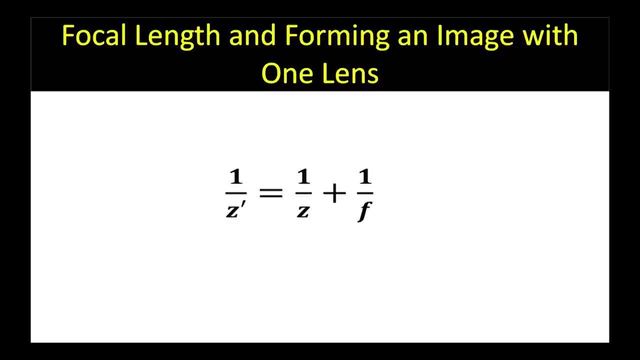 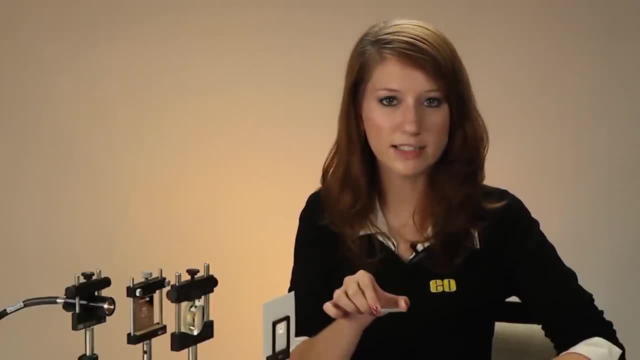 Typically we're working in air, so n and n prime both equal 1.. For this equation we're assuming the lens is thin, meaning the diameter of the lens is about 10 times larger than its thickness. Also, we use a sign convention here that dictates that we write a distance. 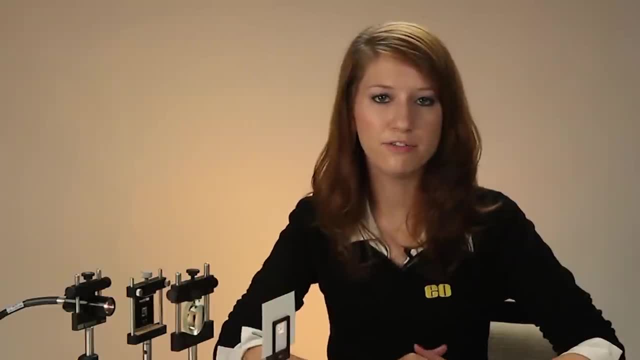 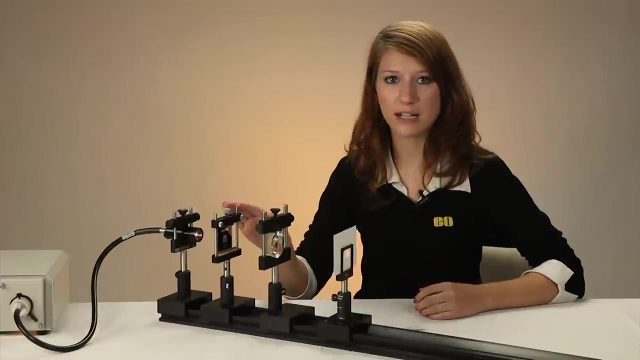 measured to the left as a negative number, so z would be negative for the case shown here. This equation governs where an image will form. You can choose any two of the variables and solve for the third when setting up your imaging system. I'd like to illustrate three different scenarios for you using this object. As you can see, 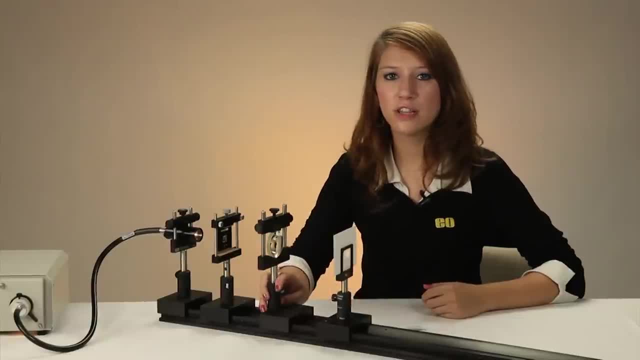 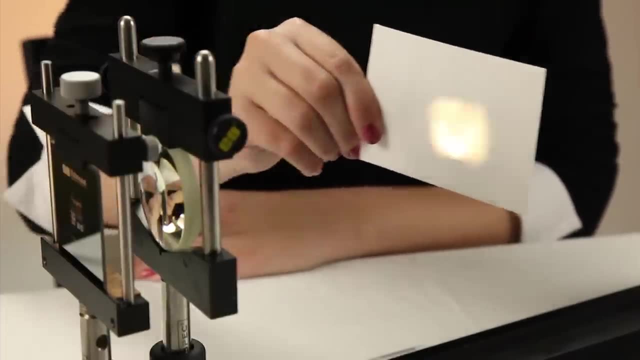 in the first setup, if the object you are trying to image is closer to the lens than the focal length of the lens, in our case 50mm, an image of the object will not form In this second setup once the lens is at least one focal length away from the object. 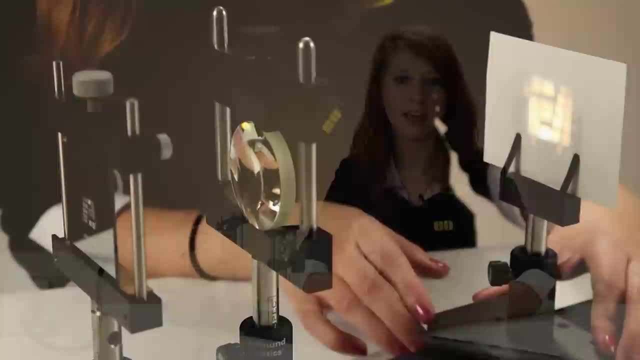 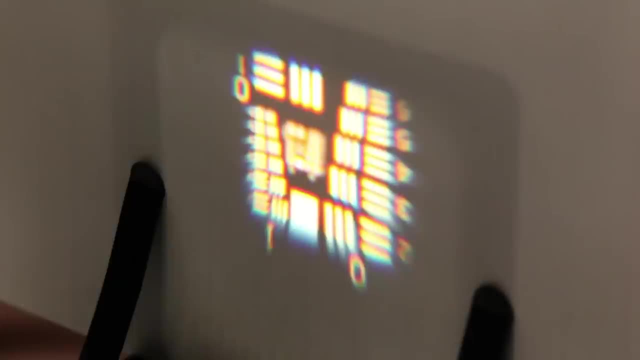 an image will form as governed by the equation I just described. In this case, we will move the lens to be 70mm from the object, so an image will form 175mm away. You can see that as we move the lens, the distance to the image also changes The light. 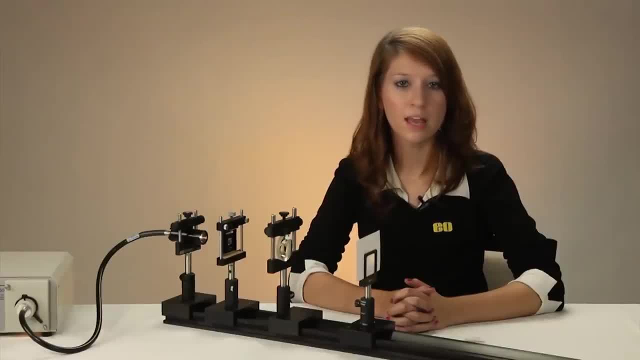 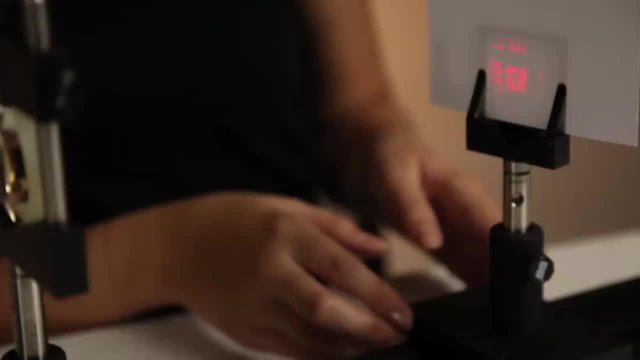 does not always focus at one focal length away from the lens. As seen in this final setup, I'm using a laser source for collimated light. Collimation means that all of the light rays are traveling parallel to each other, not continuously. That's the. 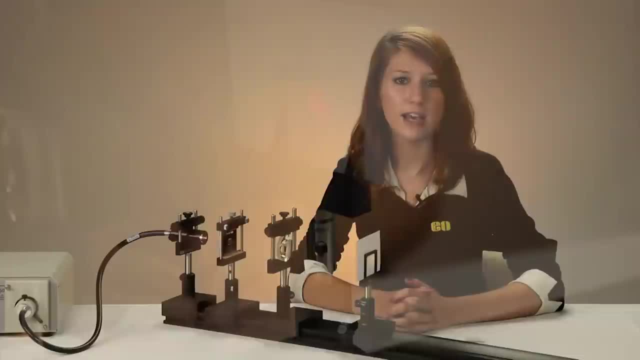 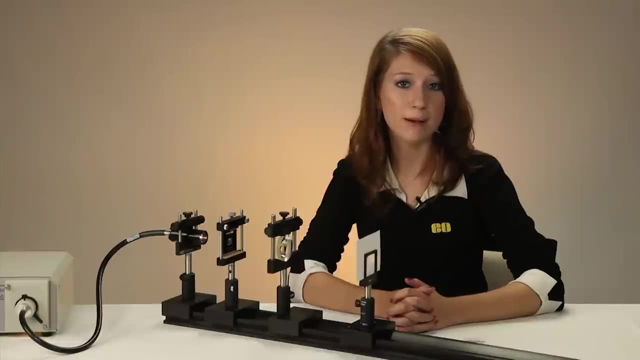 point, The image will form at a distance equal to the focal length of the lens. Once the lens is far enough away from the object- about 10 times the focal length of the lens- we can consider it to be collimated. I hope this answers some of your questions about finding the image from a single lens.